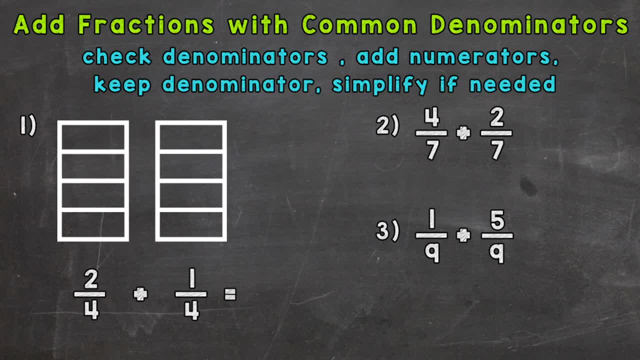 So let's jump right into number one here And we have rectangles filled with rectangles above our problem of two-fourths plus one-fourth. So that picture there that's going to help us model and visualize what's happening in this problem. So the first thing we need to do is check our denominators. 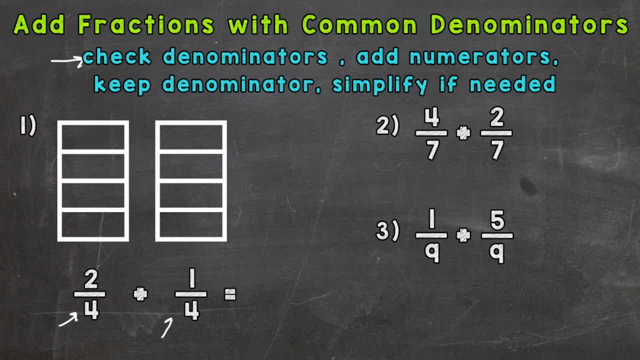 And we have a four here and a four. We need to check denominators because that's a good habit to get into when it comes to fractions, Because if you don't have common denominators in adding or subtracting fractions problems, it takes an extra step or two. 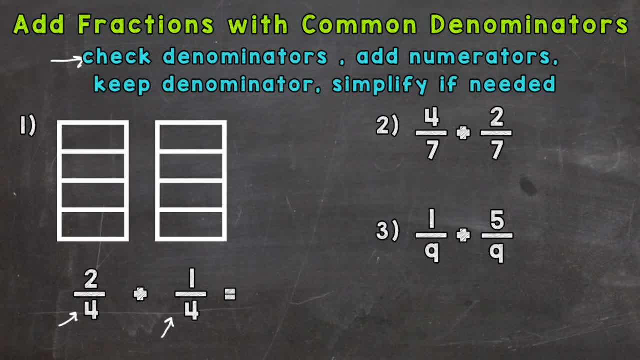 So in this case we do have a common denominator. So now we add our numerators. Our numerators are our top numbers, So two plus one gives us three. We always keep our denominator the same, So four, four, And in our answer our denominator is going to be four. 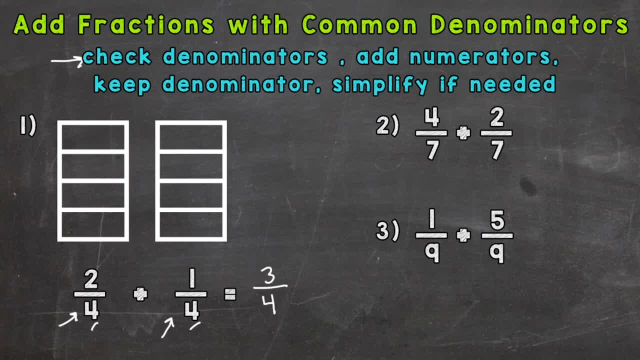 And we simplify if needed. In this case, three-fourths is already simplified. The only common factor between three and four is one. So we're in simplest form: Our answer is three-fourths. So let's do this with our model here. 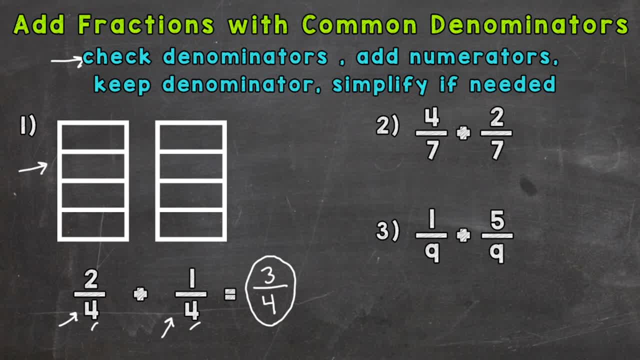 So our first rectangle here is cut into one, two, three. It's cut into fourths. So we need to fill in two-fourths to represent that two-fourths In our addition problem. One-fourth, two-fourths. And in our second rectangle we need to fill in one-fourth to represent that one-fourth in our problem. 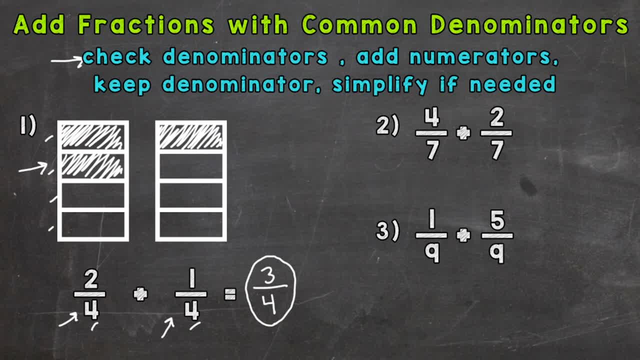 So now, how many total fourths are filled in? Well, we have one-fourth, two-fourths plus the one-fourth gives us a total of three-fourths. So we have one-fourth, two-fourths plus the one-fourth gives us a total of three-fourths. 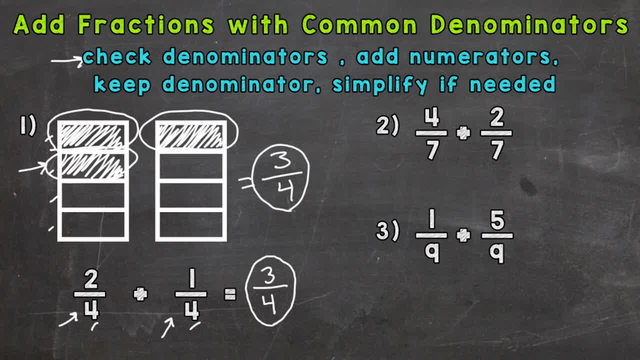 So our model matches our answer. So let's go to number two. So again, we always check our denominators And they are common denominators there or like denominators. If you hear common or like denominators, they mean the same thing.